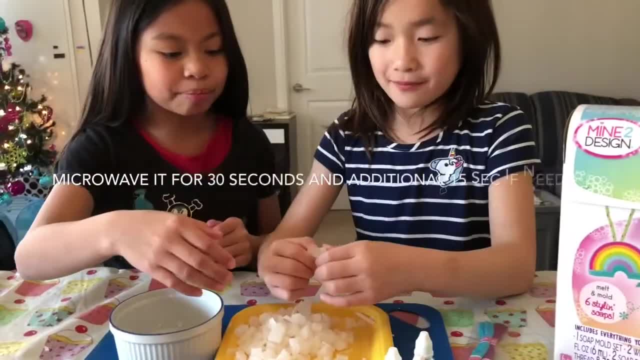 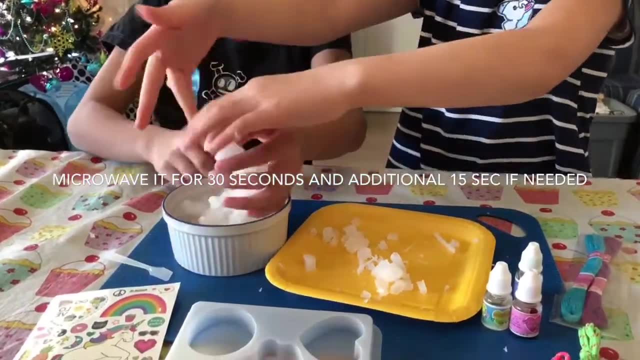 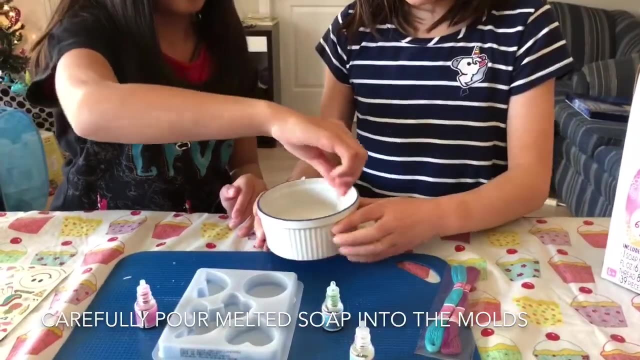 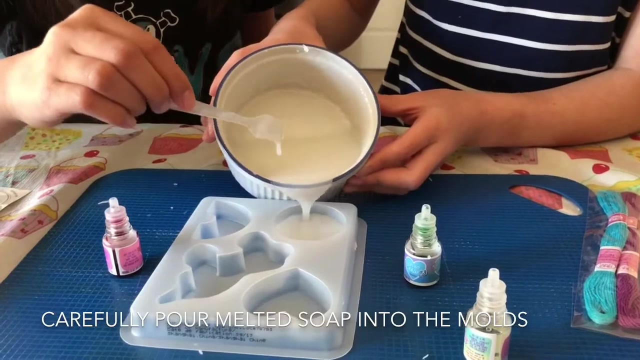 We're going to melt it in the microwave for 30 seconds. Ew sticky, I feel like it's slimy. It's raining, so it's melted and we're going to pour some in the mold. I think that's enough. No, that's enough pigeon. 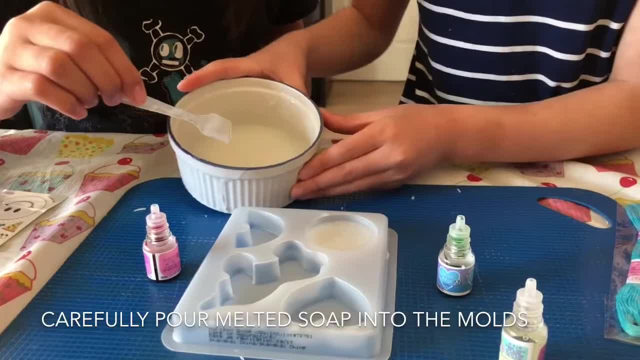 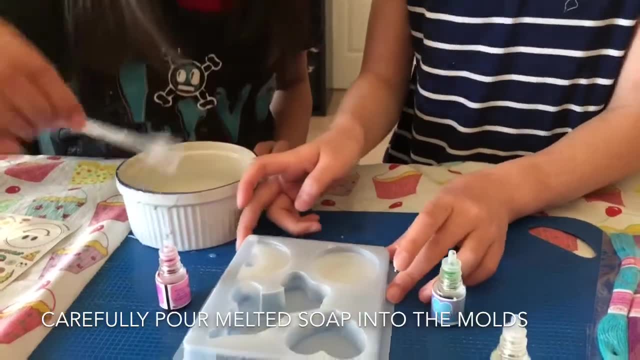 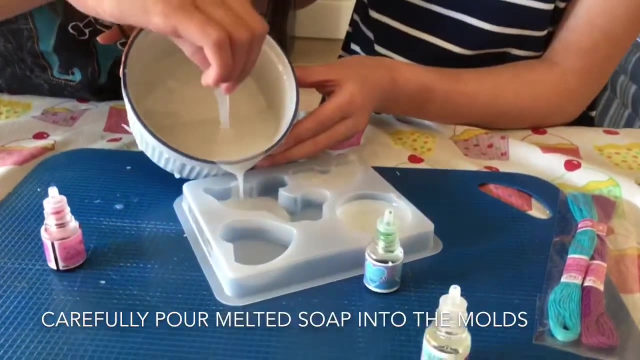 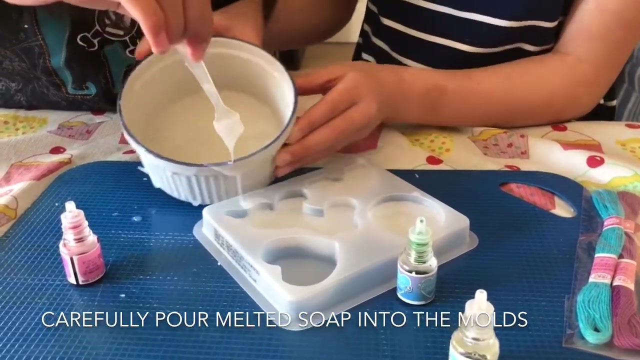 Now we're going to do the rainbow. That should be good, And that The unicorn. The unicorn is going to be the biggest one. Yeah, so we need a lot. That should be enough, right. Just a little more. That should be good, right? Oh no, it's poured out, Oh well. 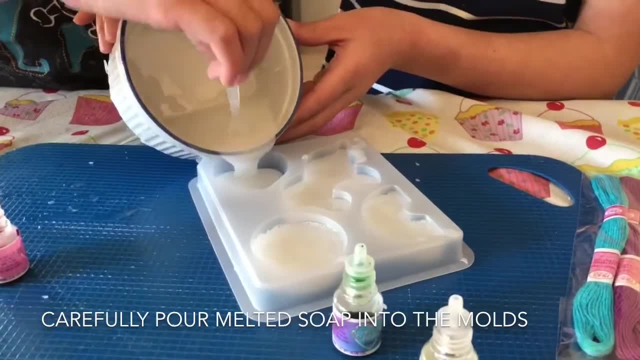 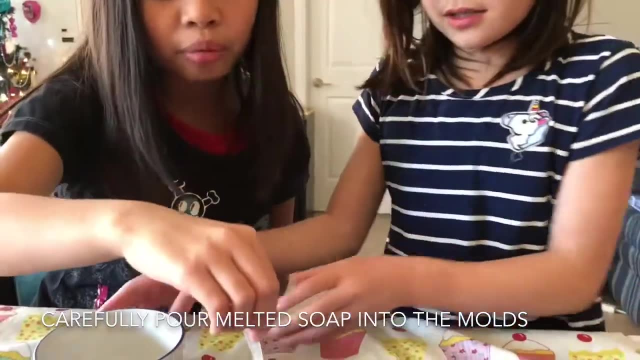 Oh well, whatever It's still going to be in shape. Nope, Oh no, we put too much, It's okay. Oh, we could have put a little more. Yeah, Just a little more. Okay, that's enough. 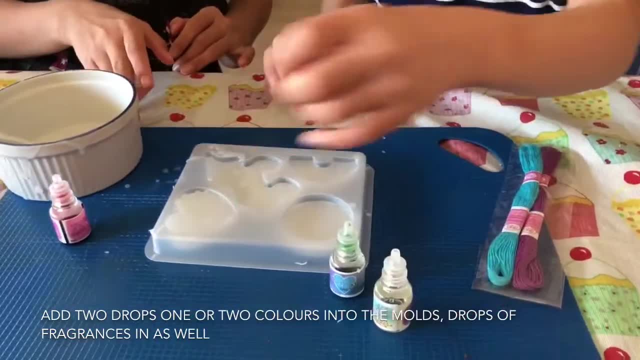 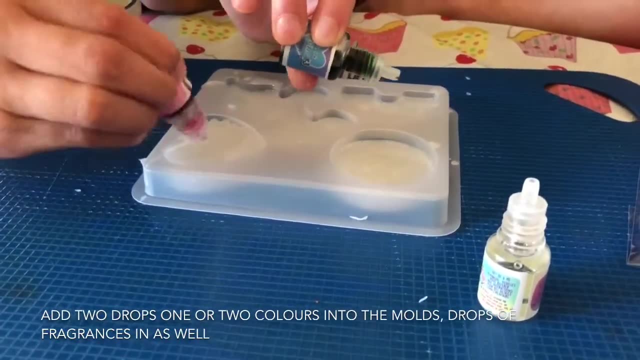 Okay, Oh no, It's okay. So now I'm going to take the green, So now I'm going to pour it. I can't squeeze it out. I can't squeeze it out, Just tilt it over. Yeah, I did. 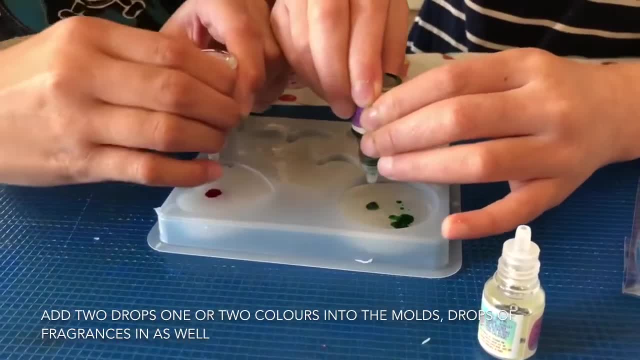 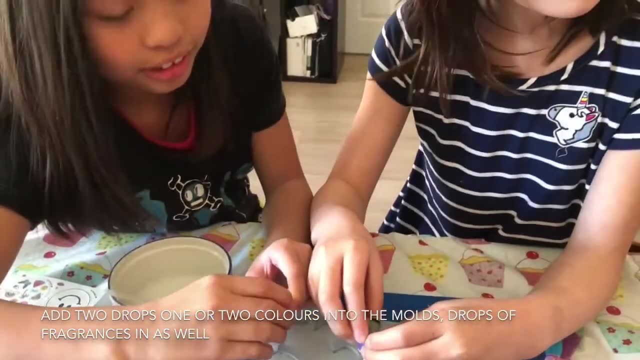 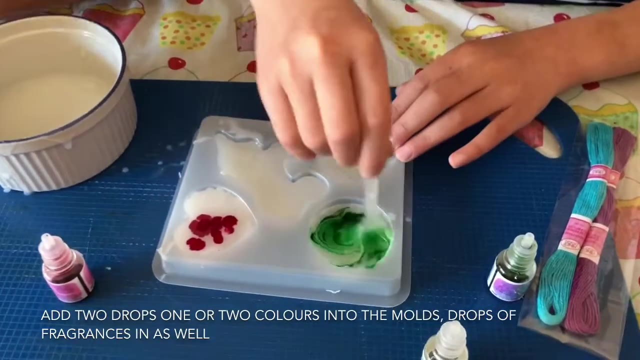 Oh, How did you do that? Oh, Should that be enough? Or a little more Mm, And now we will mix it. You'll go first for the mixing. I think you need to add a little green, I think. 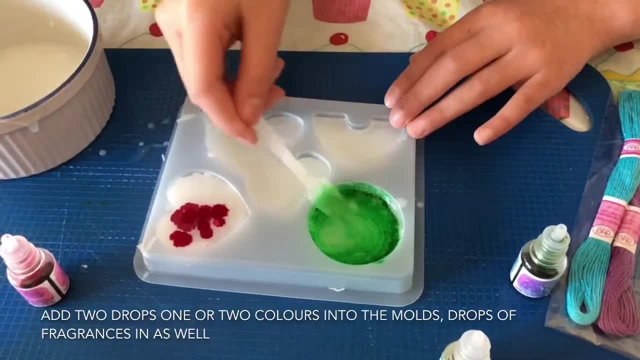 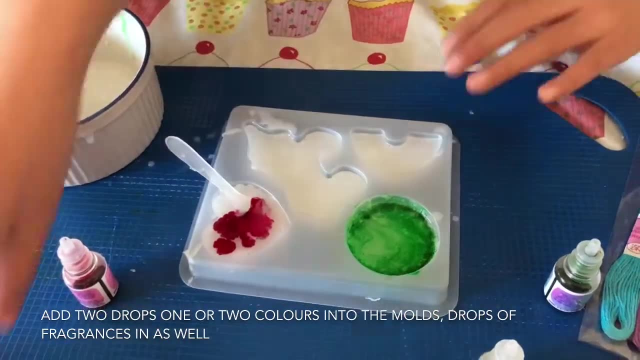 Actually. no, that's enough. That's a lot of green. Yeah, Oh, no, now we need water, because I'm going to put it in red Here. now you mix it and I'll pour in some glitter, Glitter, glitter, glitter. 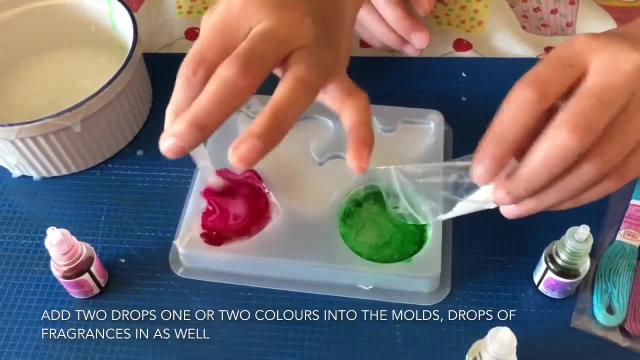 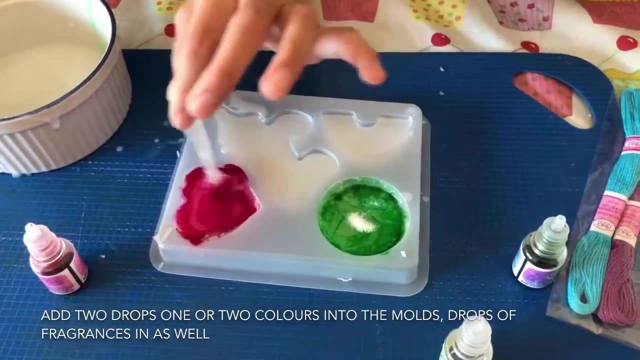 Do you think I should add a little bit more red? No, it's up to you Here, Actually. no, it's okay, And so I'm done. Mix it Okay, Okay, Okay, Okay, Okay, Okay.